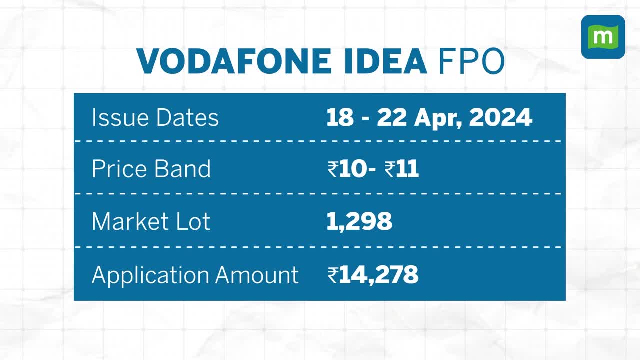 subsequent bids in the multiples thereof. That means that a minimum investment amount required by a retail investor like Aditya Birla Bank will be kept to 1,298 equity shares. This means that you and me would be 14,278 rupees. So if you were to consider the upper limit of this price band, 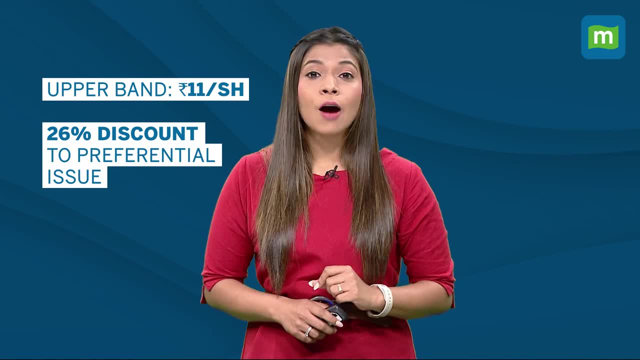 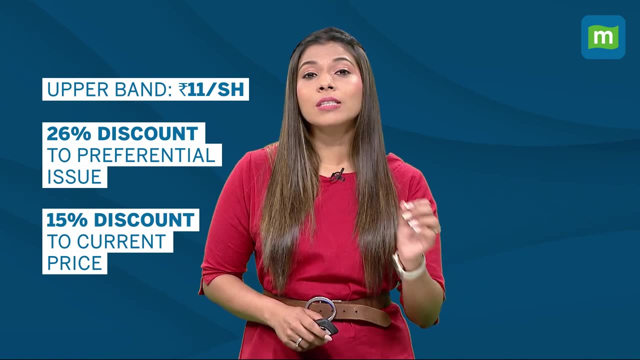 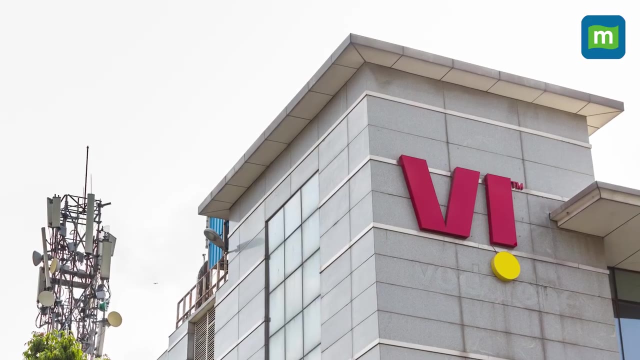 which is 11 rupees per share. it comes at a considerable discount of 26% compared to that recent preferential issue priced for the promoter entity which was at 14.87 rupees. This is also a 15% discount to the current market price of where Vodafone Idea is trading The follow-on public. 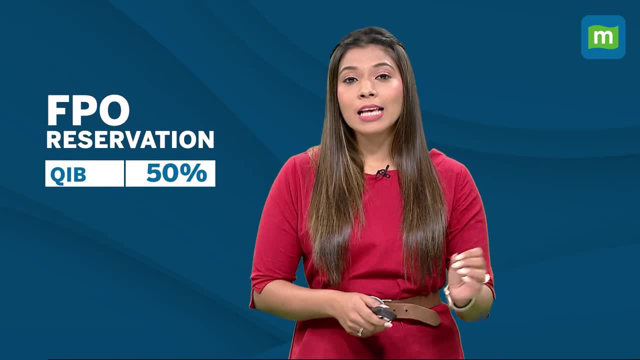 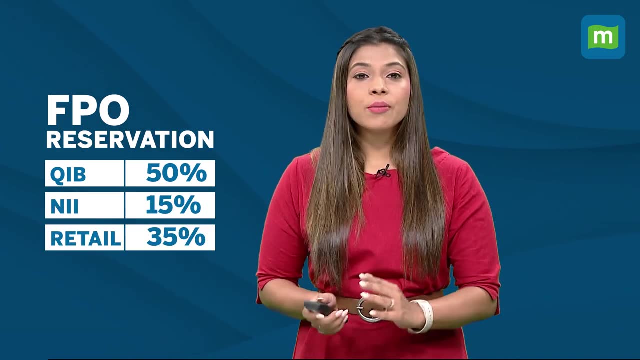 is that the current market price for the Vodafone Idea FPO is at 15.73 rupees, and that means that the current market price for the Vodafone Idea FPO is at 15.72 rupees. This means that the current market price of the Vodafone Idea FPO is at 16.62 rupees. So if you have a large stock of shares, and you have to pay 10,000 rupees for the project. then you need to pay 15,000 rupees for the project and that is the total amount which the company is going to be paying. There is a total of 15%. 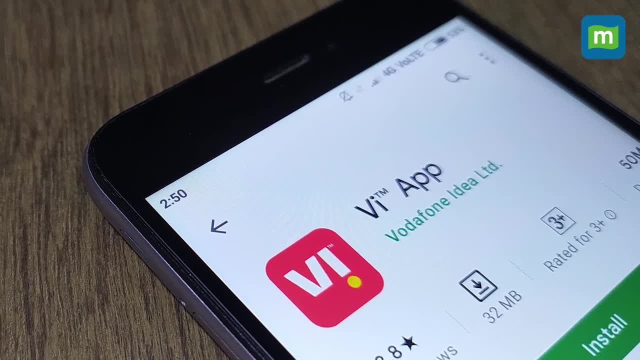 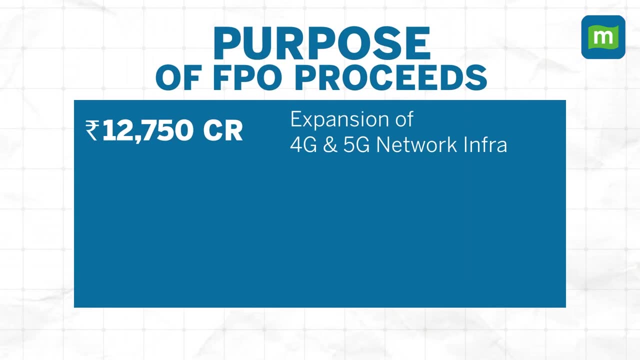 for the project and the remaining 35% for the retail investors. So where exactly does Vodafone plan to use this money? Over the total FPO proceeds, the telco proposes to use about 12,750 crores for the purchase of equipment for the expansion of the network infrastructure by setting up a new 4G site. 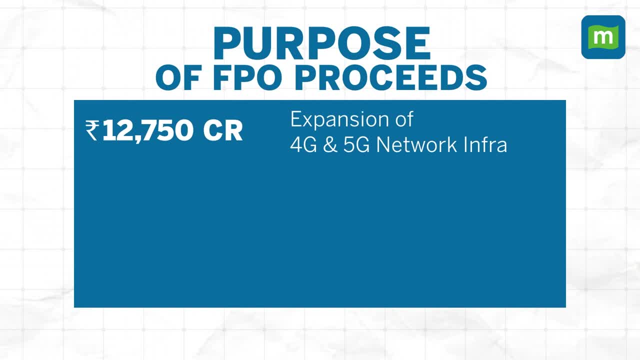 looking to expand the capacity of the existing 4G sites and also setting up new 5G sites. now 2175.31 crore rupees from the FPO proceeds has also been set aside for the deferred payments of spectrum to the Department of Telecom. as 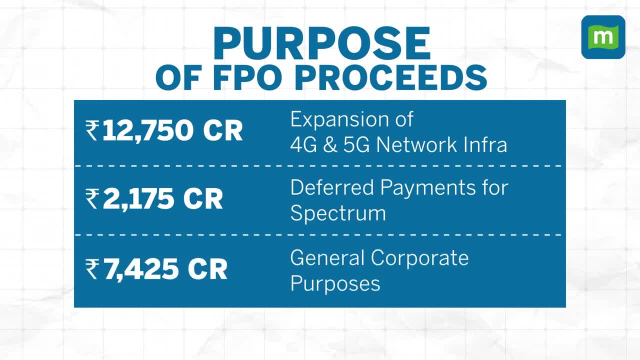 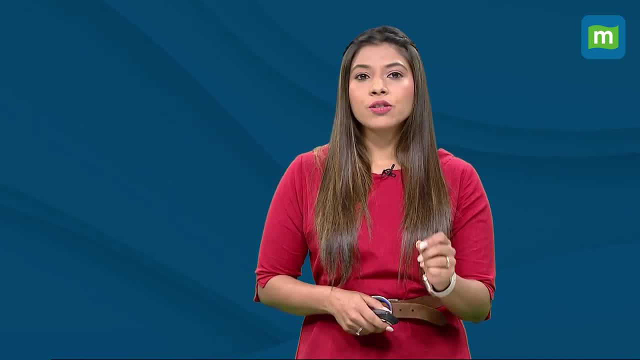 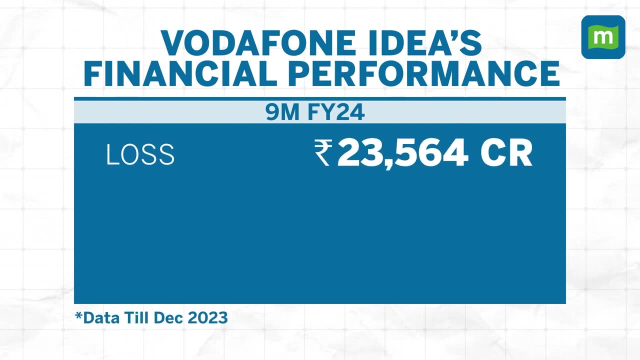 well as GST. the remaining funds will be used for general corporate purposes, but is this enough for you to consider entering the stock via the FPO route? see, going by the financials, the company incurred a loss of about 23 thousand five hundred sixty four crore rupees in the nine months ending December 31st of. 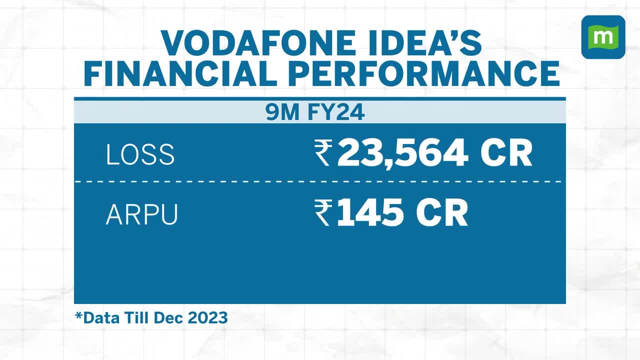 2023, whereas the average revenue per user- or are fool that one- rose just about 245 rupees, which, when compared to Gio, its biggest competition, came at about 181 point seven rupees. and if we were to look at the total debt of the company as